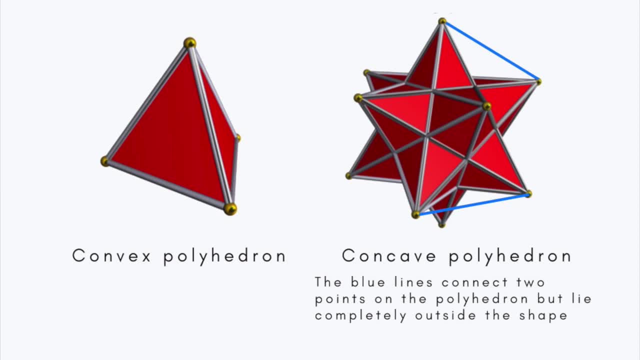 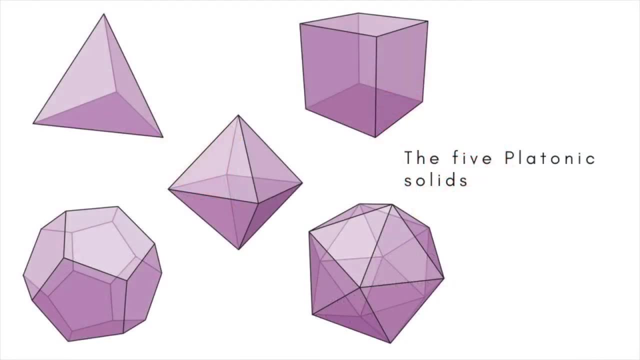 is completely inside or on the polyhedron, the figure is convex. Otherwise it's concave. A polyhedron is regular if all of its faces are exactly the same size and shape and if the same number of faces meet at each vertex. There are only five regular convex. 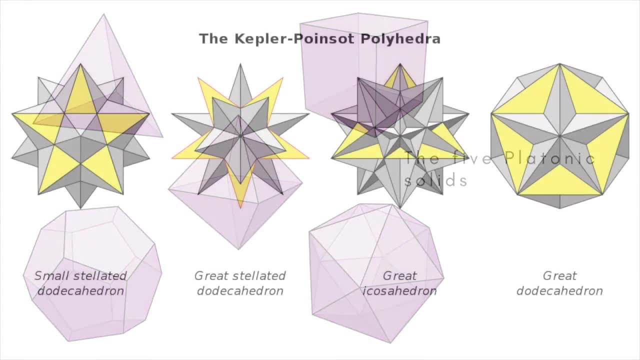 polyhedrons, the platonic solids. A further four regular polyhedrons, the so-called Kepler-Poiseau solids, exist that are non-convex. However, the term regular polyhedrons is sometimes used to describe only the platonic solids. 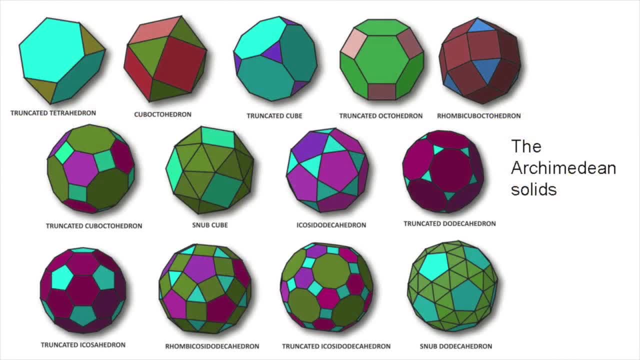 A convex polyhedron is said to be semi-regular if its faces have a similar arrangement of non-intersecting, regular plane convex polygons of two or more different types about each vertex. These solids, of which the polyhedron is a regular polyhedron, are non-convex. 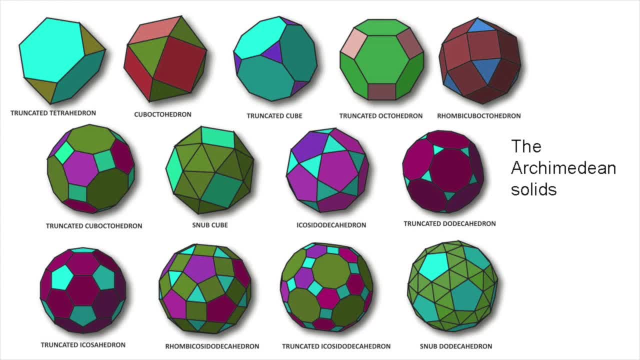 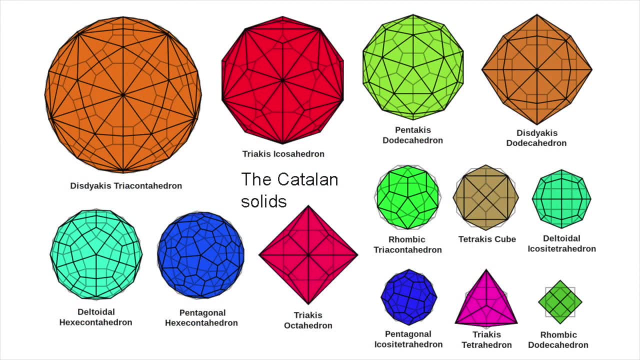 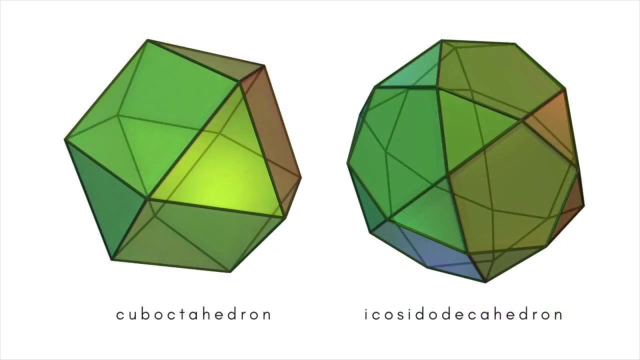 A dual of a polyhedron is another polyhedron in which faces and vertices occupy complementary locations. The duals of the Archimedean solids are known as the Catalan solids. A quasi-regular polyhedron is the solid region interior to two dual regular polyhedrons. 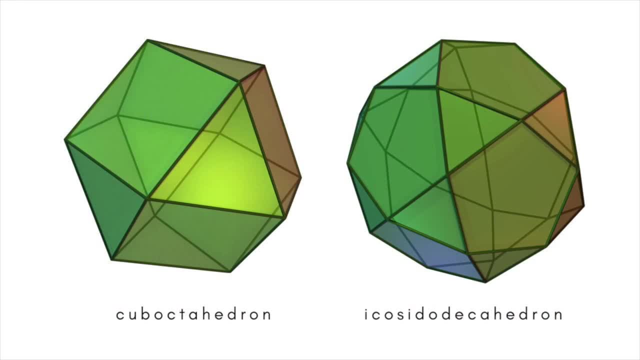 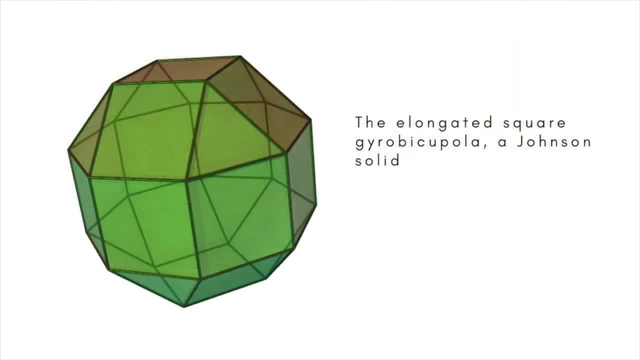 Only two exist: the cuboctahedron and the icosidodecahedron. There are also infinite families of prisms and antiprisms which, like the Archimedean solids, are considered to be semi-regular if all their faces are regular polygons In 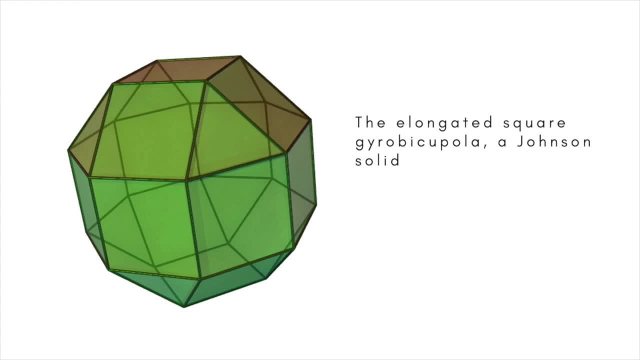 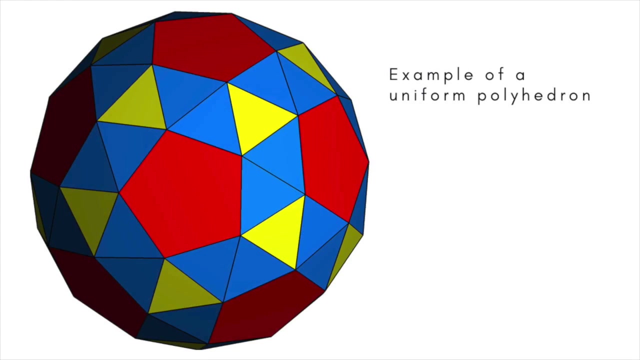 total, there are ninety-two convex polyhedrons with regular polygonal faces and not necessarily non-convex polyhedrons. The uniform polyhedron is a polyhedron in which each face is regular and each vertex is equivalently arranged. Uniform polyhedrons include the platonic solids, the Archimedean, 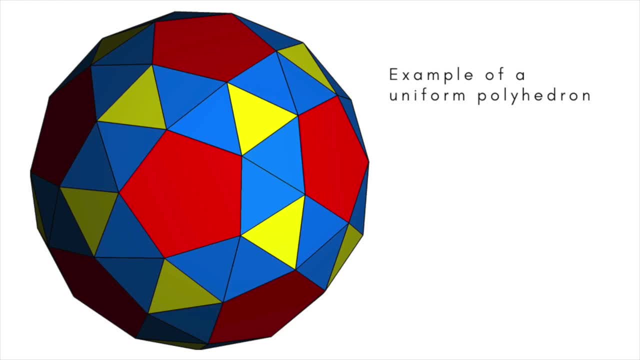 solids and the concave uniform polyhedrons. The uniform polyhedron is a uniform solid with uniform vertex and non-concave polygonal faces. The uniform polyhedron is a uniform solid with uniform vertex and non-convex polygonal faces. 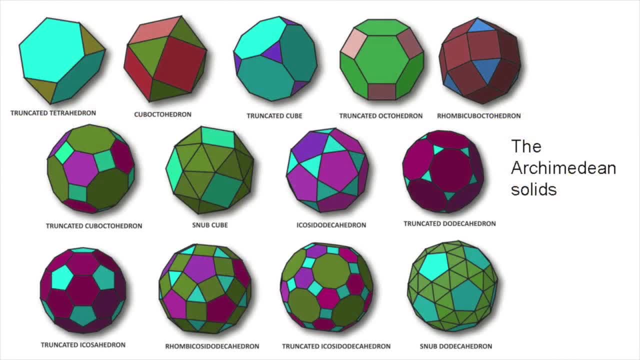 A convex polyhedron is said to be semi-regular if its faces have a similar arrangement of non-intersecting, regular plane convex polygons of two or more different types about each vertex. These solids, of which the polyhedron is a regular polyhedron, are non-convex. 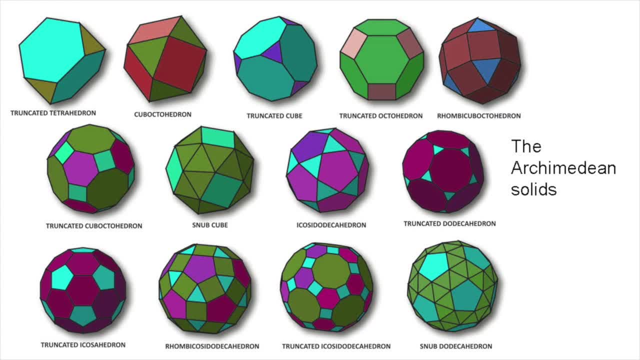 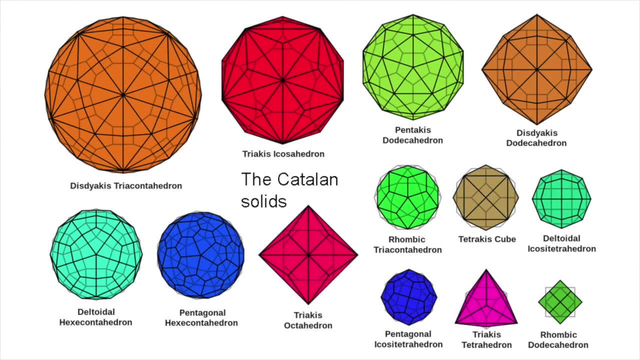 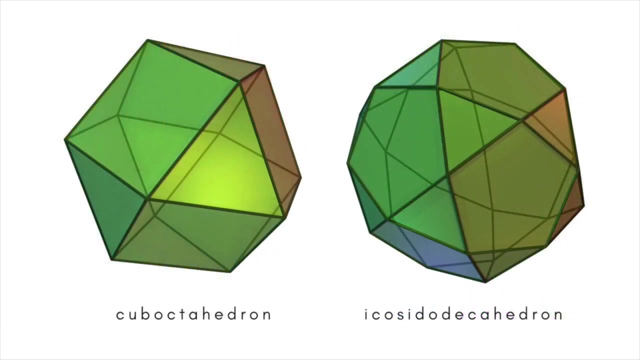 A dual of a polyhedron is another polyhedron in which faces and vertices occupy complementary locations. The duals of the Archimedean solids are known as the Catalan solids. A quasi-regular polyhedron is the solid region interior to two dual regular polyhedrons. 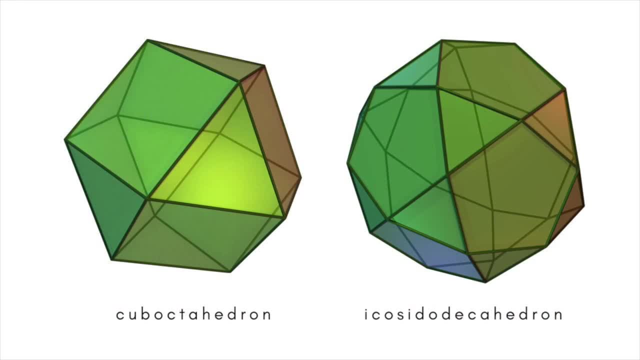 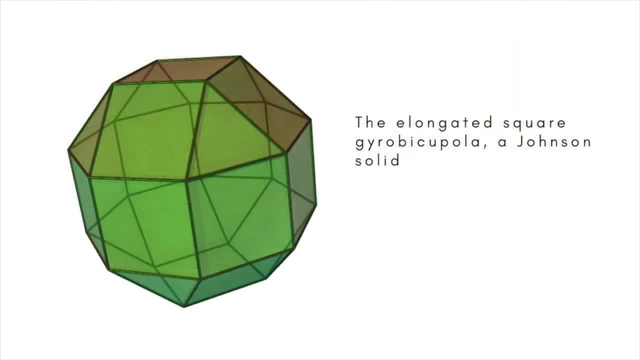 Only two exist: the cuboctahedron and the icosidodecahedron. There are also infinite families of prisms and antiprisms which, like the Archimedean solids, are considered to be semi-regular if all their faces are regular polygons In 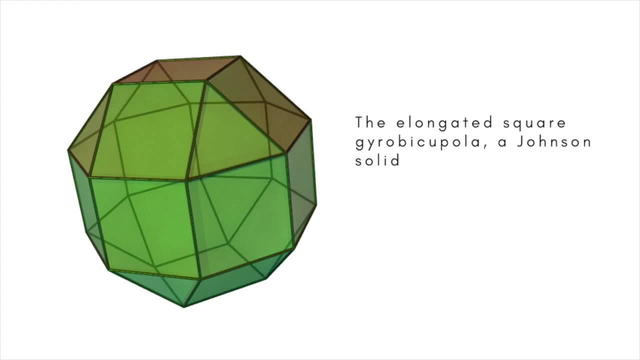 total, there are ninety-two convex polyhedrons with regular polygonal faces and not necessarily regular polyhedrons. These are the Johnson solids. The third is a uniform polyhedron in which faces are regular and each vertex is equivalently arranged. 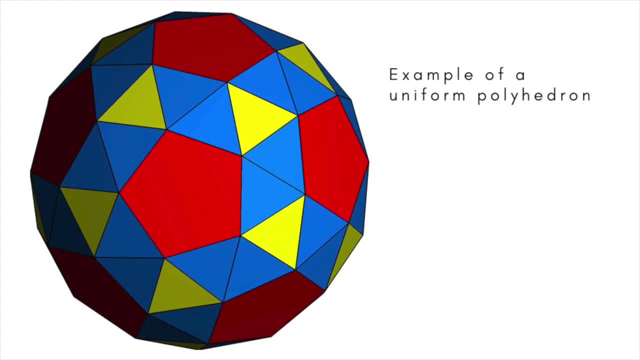 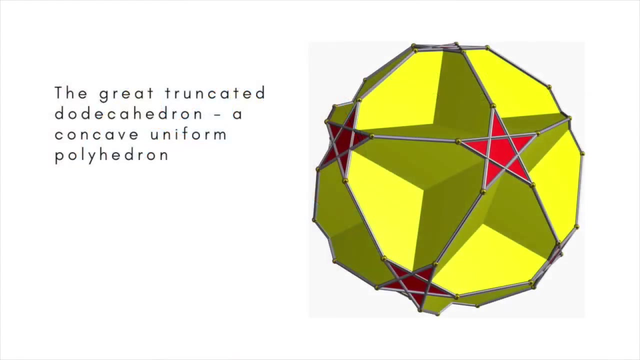 A uniform polyhedron is a polyhedron in which face is regular and each vertex is equivalently arranged. Uniform polyhedrons include the platonic solids, the Archimedean solids, the prisms and antiprisms and the concave uniform polyhedrons. 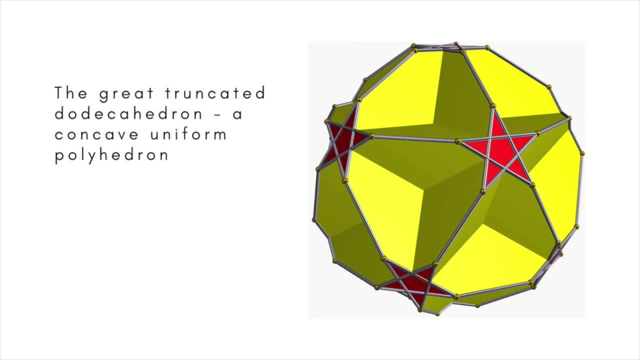 Uniform polyhedron is a uniform polyhedron of a type obtained by relaxing the conditions used to produce the Archimedean solids, which have regular convex faces and identical convex vertices to allow both non-convex faces and vertex types, as in the case of the Kepler-Poiseau. 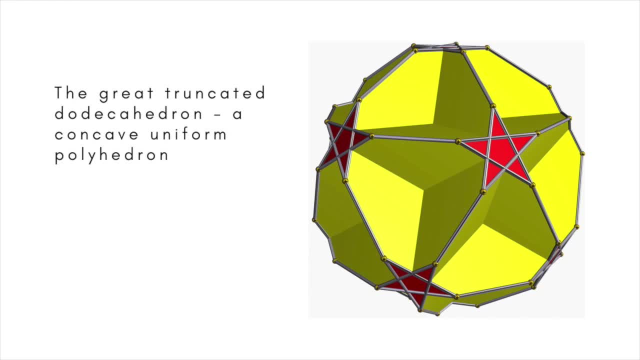 solids. The condition that every vertex must be identical but the faces need not be gives rise to 53 non-convex uniform polyhedrons. An example is the great truncated dodecahedron, obtained by truncating the corners of the 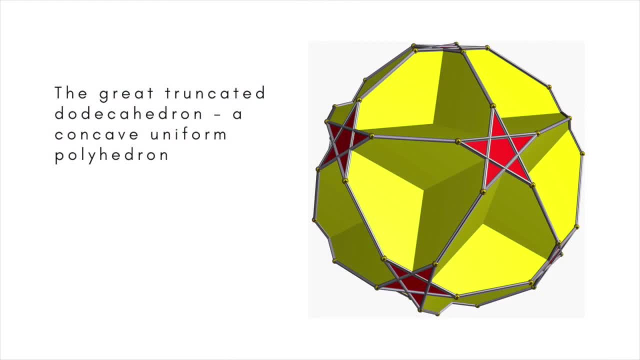 These vertices are the learning object of an archimedean solid is a uniform polyhedron of a type obtained by relaxing the conditions used to produce the Archimedean solids, which have regular convex faces and identical convex vertices to allow both non-convex faces and vertex types, as in the case of the Kepler-Poiseau solids. 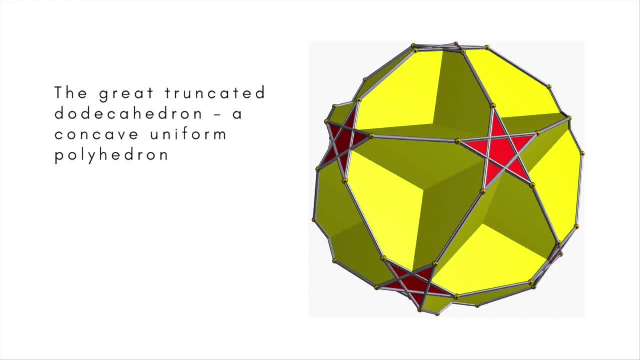 The condition that every vertex must be identical but the faces need not be gives rise to 53 non-convex uniform polyhedrons. An example is the great truncated dodecahedron, obtained by truncating the corners of the great dodecahedron at a depth which gives regular decagons. 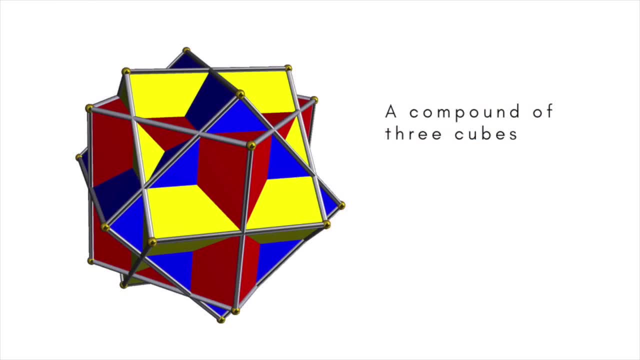 A compound polyhedron is an assemblage of two or more polyhedrons, usually interpenetrating and having a common centre. There are two types: a combination of a solid with its dual and a combination of a solid with its dual. A compound polyhedron is an assembly of two or more. 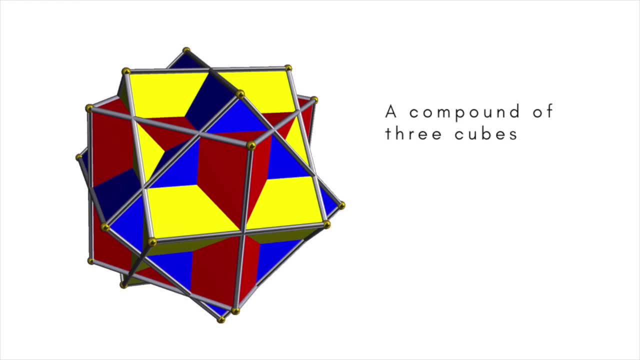 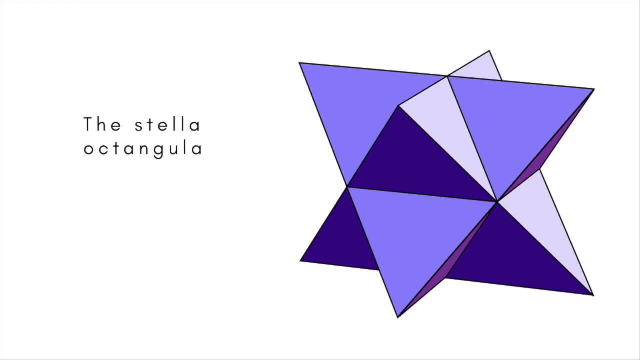 polyhedrons and an interpenetrating set of several copies of the same polyhedron. The simplest example of a compound polyhedron is the compound of two tetrahedrons, known as the stellar octangular and first described by Johann Kepler. This shape is unique in that it falls under 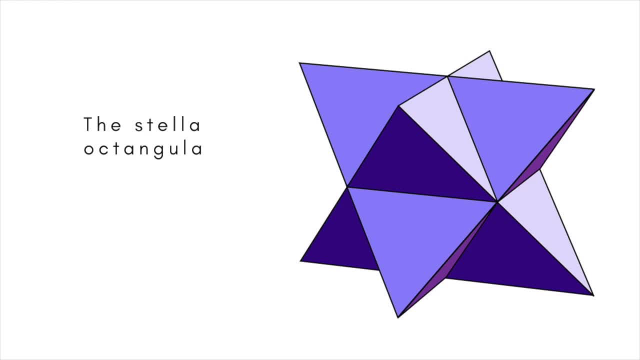 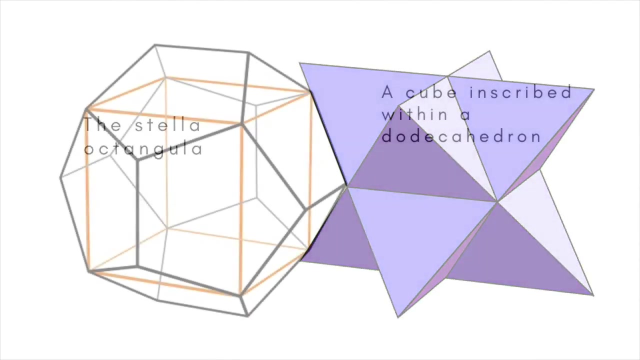 both of the above classes, because the tetrahedron is the only self-dual uniform polyhedron. The edge of the two tetrahedrons form the diagonals of the faces of a cube in which the stellar octangular can be inscribed. Another example of a compound polyhedron follows from an important platonic. 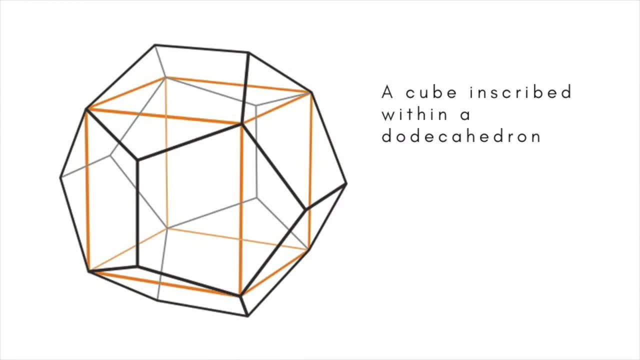 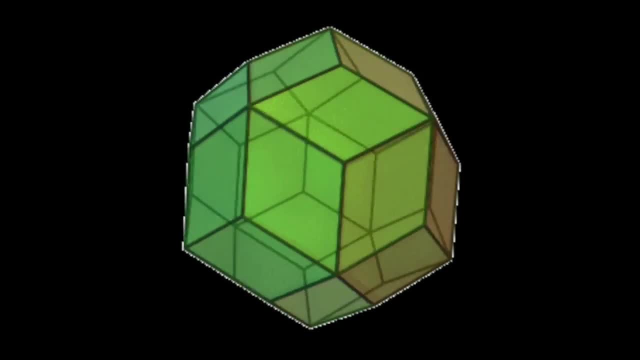 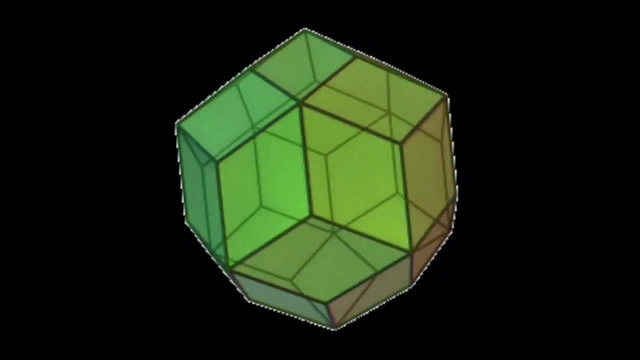 relationship. A cube can be inscribed within a dodecahedron. There are five different positions for a cube within a dodecahedron. Superimposing all five gives the compound polyhedron a shape known as the rhombic triacontahedron, The oldest known examples of human-made 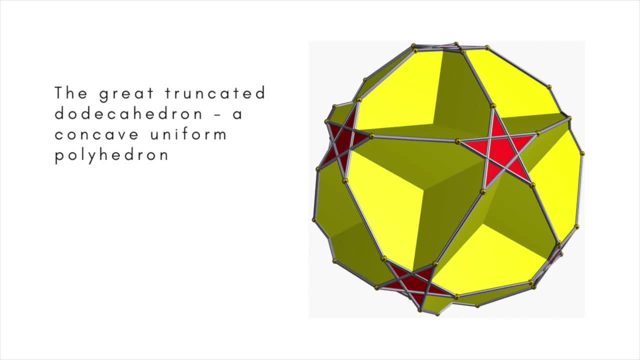 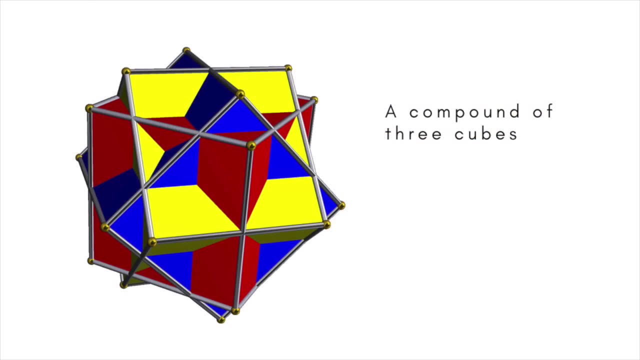 great dodecahedron at a depth which gives regular decagons. A compound polyhedron is an assemblage of two or more polyhedrons, usually interpenetrating and having a common centre. There are two types: A combination of a solid with its dual. 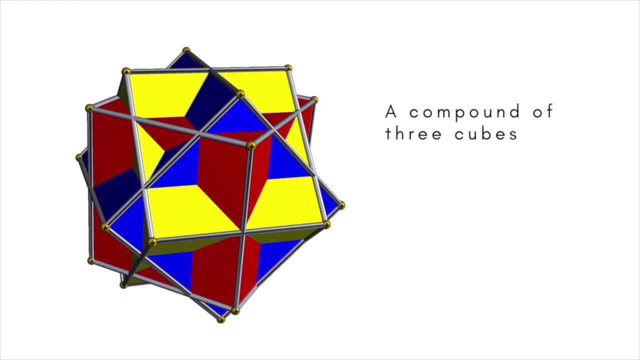 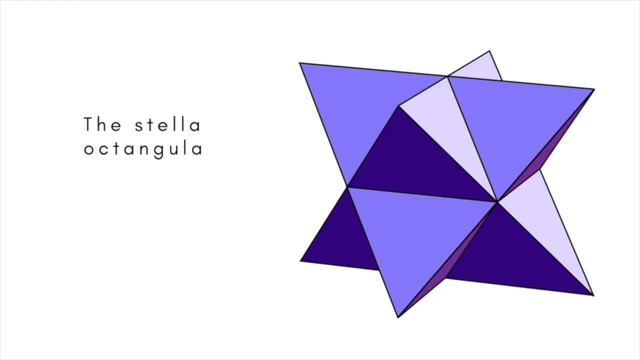 and an interpenetrating set of several copies of the same polyhedron. The simplest example of a compound polyhedron is the compound of two tetrahedrons known as the stellar octangular and first described by Johann Kepler. This shape is unique in 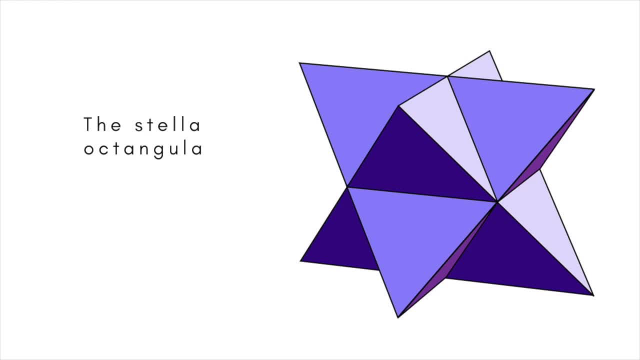 that it falls under both of the above classes, because the tetrahedron is the only self-dual uniform polyhedron. The edges of the two tetrahedrons form the diagonals of the faces of a cube in which the stellar octangular can be inscribed. 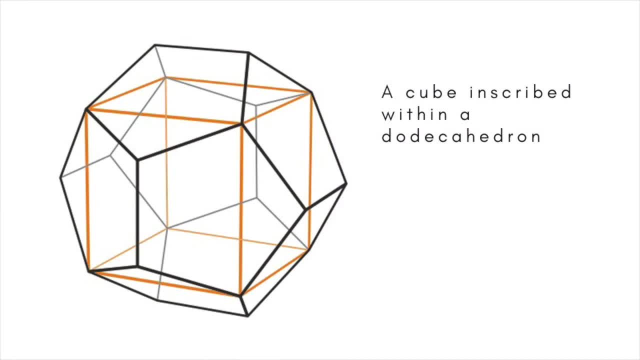 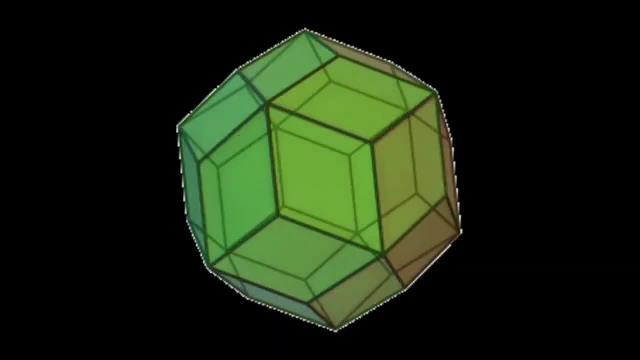 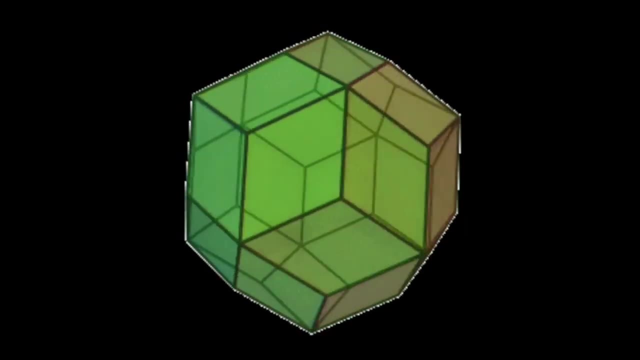 Another example of a compound, polyhedron, follows from an important platonic relationship. A cube can be inscribed within a dodecahedron. There are five different positions for a cube within a dodecahedron: 1., 2.. 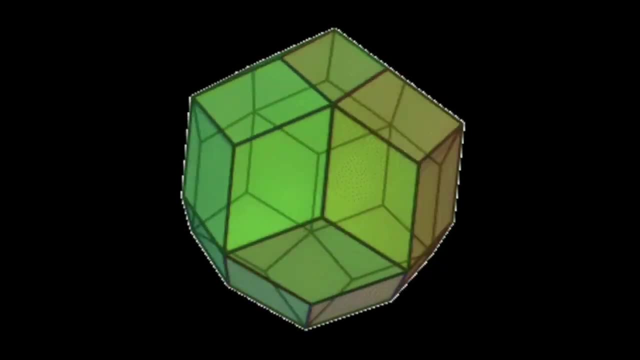 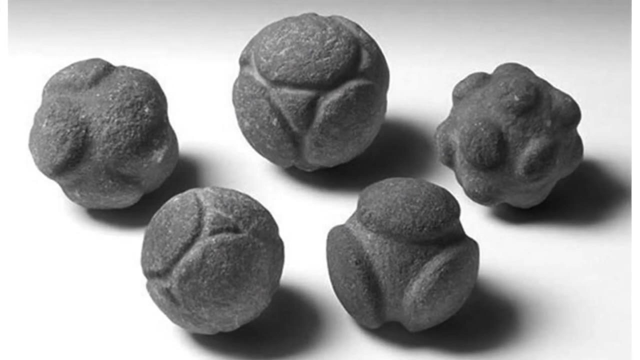 3., 4., 5., 6., 7., 8., 9., 10., 11., 12., 13., 14., 15., 16., 17., 18., 19.. 20., 21., 22., 22., 23., 24., 25., 26., 27., 28., 29., 30., 31., 22., 24., 25., 26.. 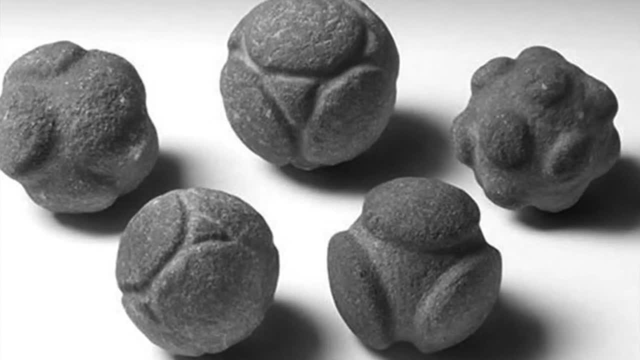 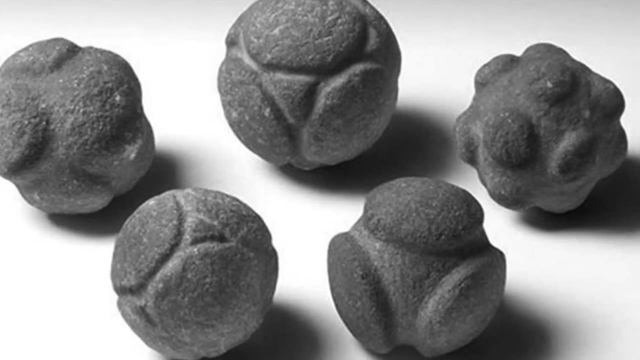 26. 27., 28., 29., 30., 31., 32., 33., 34., 35., 36., 36., 37., 38., 39., 40., 41.. 42., 43., 44., 45., 46., 47., 48..